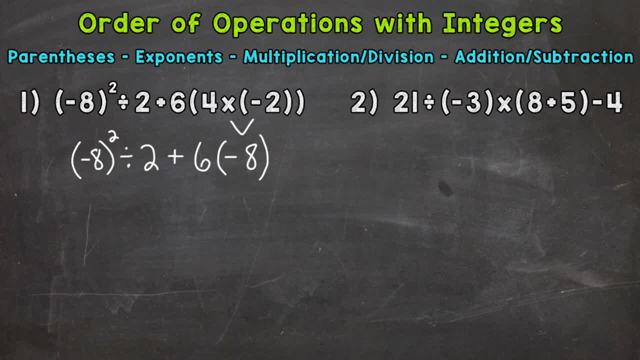 within the parentheses: No, Any exponents. Yes, So that's what we do. next We have negative eight squared. That does not mean negative eight times two, It means negative eight times negative eight. So a negative times a negative equals a positive. So we get 64.. 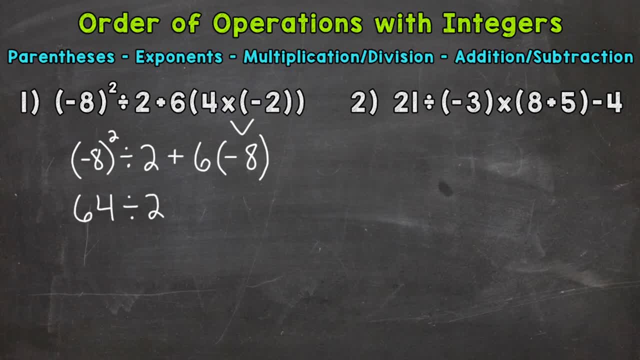 It means we do exactly the same thing over and over, and, over and over again. All right, So we have the answer given. So let's pay attention to the last thing. Do we have any parentheses? No, Any exponents, No Any multiplication or division. Yes, We have both. 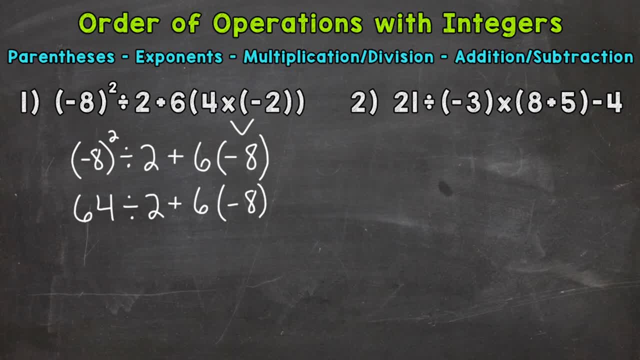 64 divided by two, and then six times negative eight. Whenever you have a number right up against parentheses, It means multiplication. Now, multiplication and division are not the same. Well, they are, And one thing you don't have to know about multiplication is that multiplication and division are very similar. 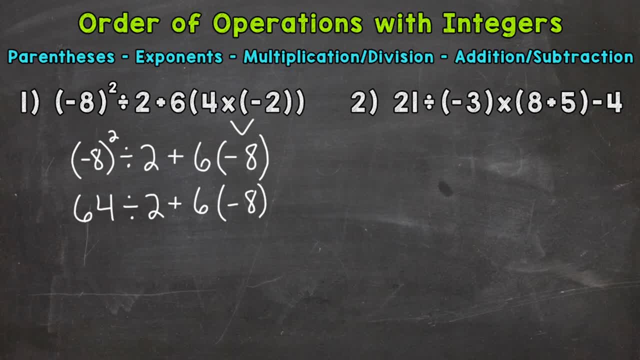 and division are on the same level, so to speak. so we solve from left to right. so 64 divided by 2 comes first. that's going to give us 32. bring down everything we did not use. so any parentheses with something inside that we need to solve. no, any exponents, no multiplication. 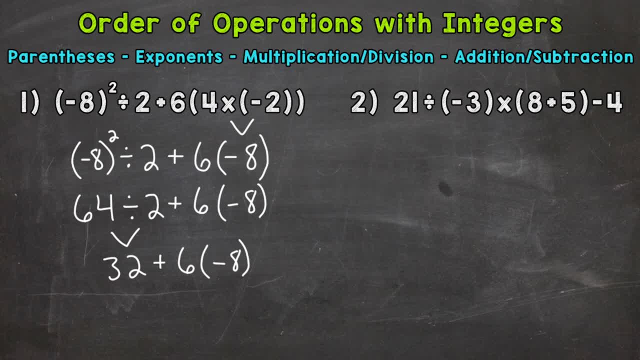 or division. yes, we have 6 times negative 8, so a positive 6 times a negative 8. that's going to give us a negative answer. so negative 48, bring down the addition sign and the 32 and we wrap things up with 32 plus negative 48. that's going to give us a negative 16 for our final answer. 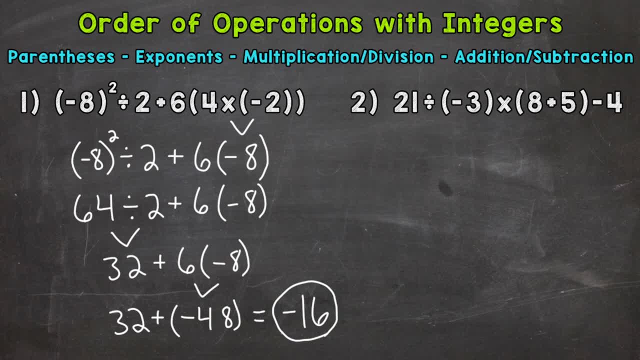 so let's move on to number two, where we have 21 divided by negative, 3 times parentheses, 8 plus 5 and parentheses minus 4. let's go through our process. so any parentheses where we have something to solve within those parentheses. yes, that 8 plus 5. so we're going to start there. 8 plus 5 is 13. 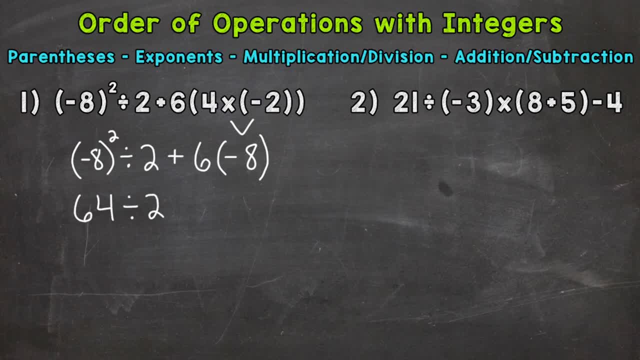 So we're breaking this problem down step by step in order to get to that final answer. So our process here: do we have any parentheses? No, Any exponents. No Any multiplication or division. Yes, we have both: 64 divided by 2 and then 6 times negative 8.. Whenever you have a 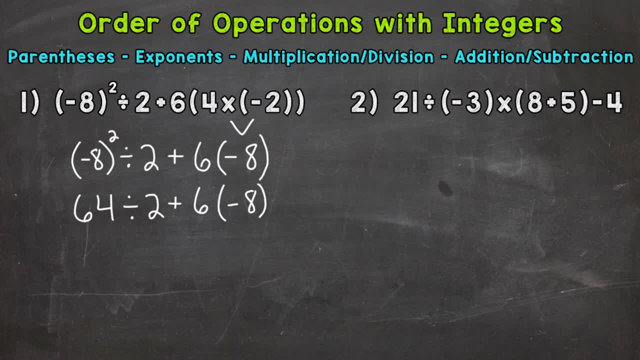 number right up against parentheses. it means multiplication. Now multiplication and division are on the same level, so to speak. so we solve from left to right. So 64 divided by 2 comes first. That's going to give us 32.. Bring down everything we did not use. 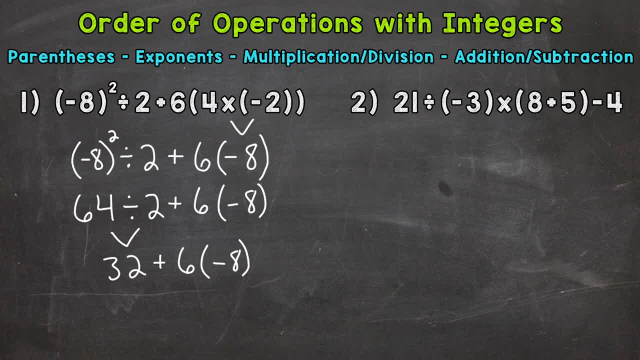 So any parentheses with something inside that we need to solve? No, Any exponents, No Multiplication or division. Yes, we have 6 times negative 8.. So a positive 6 times a negative 8, that's going to give us a negative answer. So negative 48.. 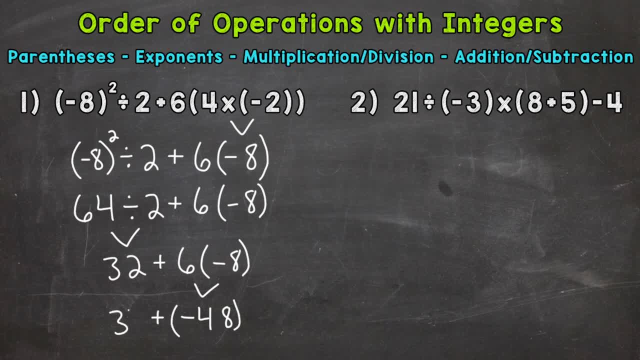 Bring down the addition sign and the 32.. And we wrap things up with 32 plus negative 48. That's going to give us a negative 16 for our final answer. So let's move on to number 2, where we have 21 divided by negative 3 times. 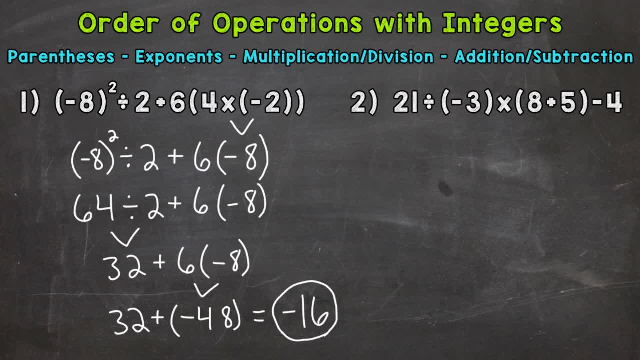 parentheses 8 plus 5 and parentheses minus 4.. Let's go through our process. So any parentheses where we have something to solve within those parentheses: Yes, that 8 plus 5.. So we're going to start there. 8 plus 5 is 13.. Bring down everything. 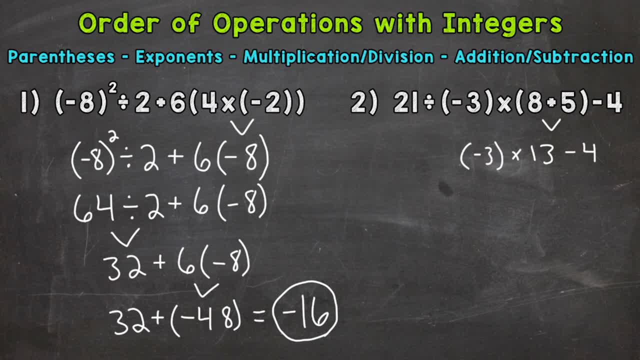 we did not use. Now keep everything in the same exact order, All right. Any parentheses where we have something to solve: No, Any exponents. No, Any multiplication or division. Yes, we have both. So solve from left to right. We will do 21 divided. 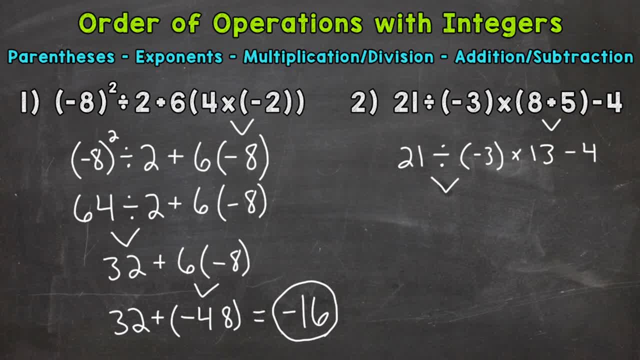 by negative 3. So we have a positive divided by a negative. That's going to give us a negative result. So we have negative 7 here I'll put it in parentheses to help organize our problem And then bring down everything we did not use.